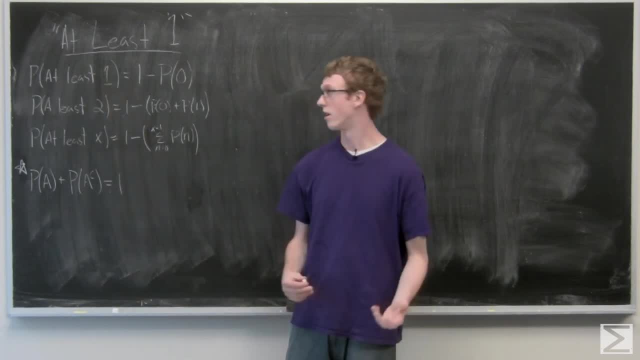 So the probability that at least that an event occurs at least once or that we get at least one success, is normally what we're looking at- success and failures here. The probability that we get at least one success is equal to one, minus the probability that we get no successes. 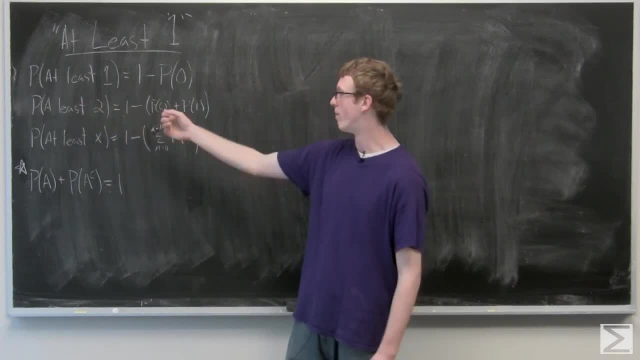 We're going to take a look at. probability of at least two is one minus the sum of zero and one success, And we can define that to the general case. The probability of at least x is going to be one minus the summation from n equals zero to x minus one. 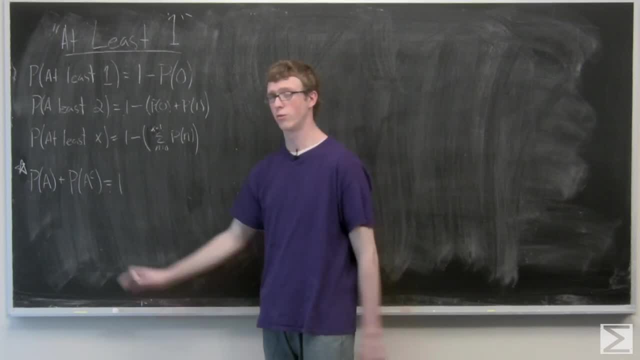 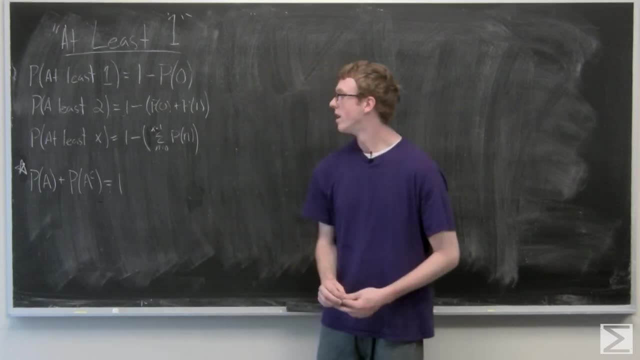 The probability of n successes. So the golden rule to remember here is going to be that the probability of a plus the probability of not a or the complement event is going to be one. So basically, what we're looking at is probability of a is one minus one. 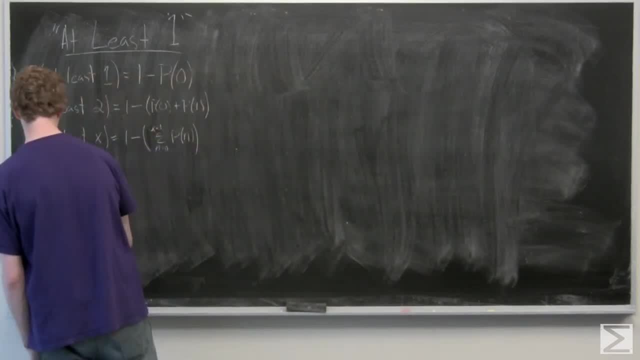 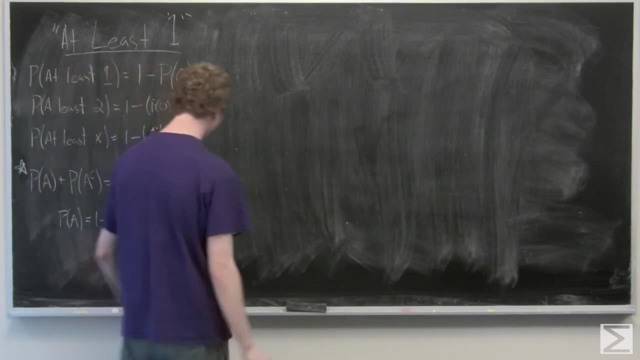 The probability of a is one minus probability of not a. Now we're most often going to be looking at successes and failures, So basically, what we're going to do is just take a look at some examples and see how this applies And then later, when we're looking at in the next video, when we're looking at Bernoulli trials and the use of binomial probability, 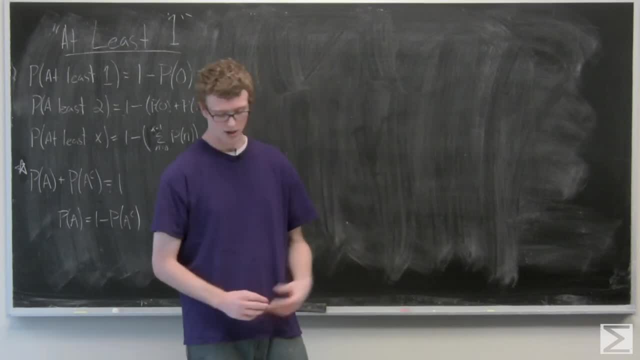 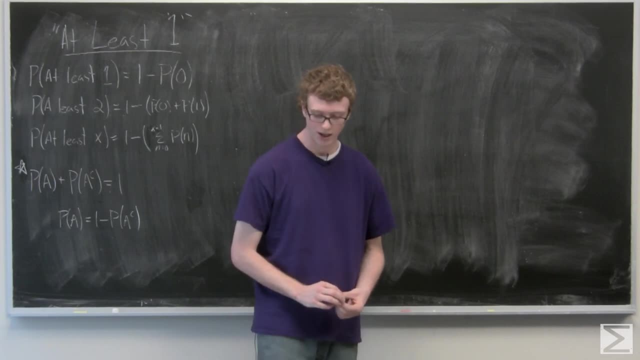 We're going to see how this can be changed. We're going to be taking a little bit further. So the first example we have states there are three reactors in a chemical plant, Each independent of the other and each of which has a 90% chance of running when an experiment begins. 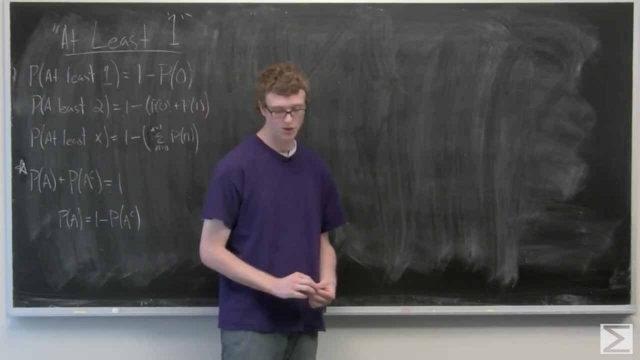 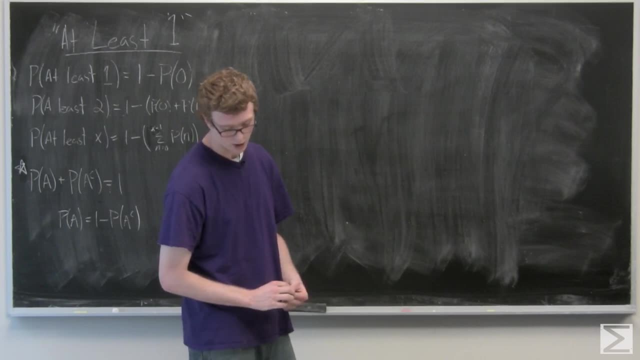 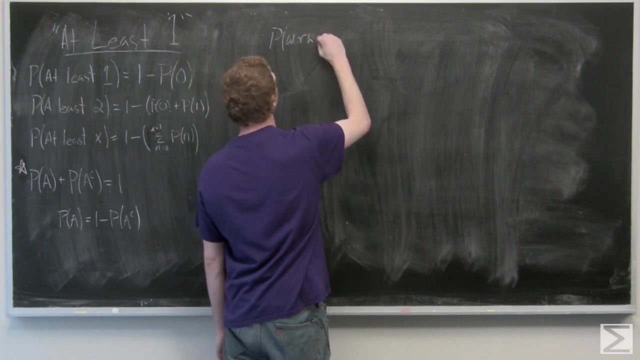 The experiment needs at least one reactor to work. So what is the probability that at least one reactor works? So we have: the probability of a reactor working is 90% or 0.9.. And we want the probability that at least one of them works. 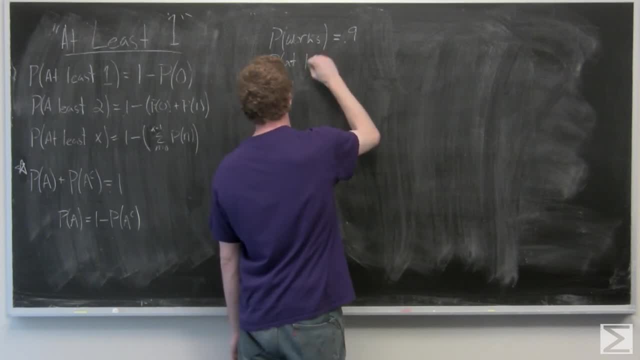 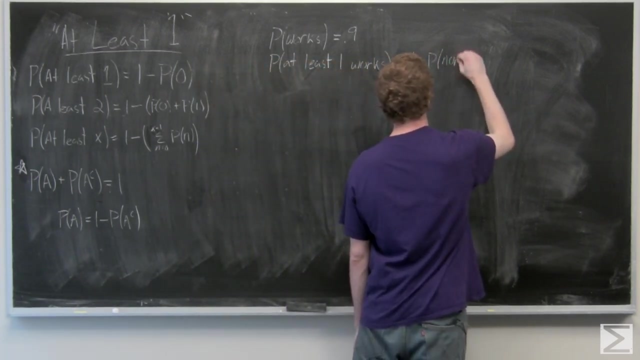 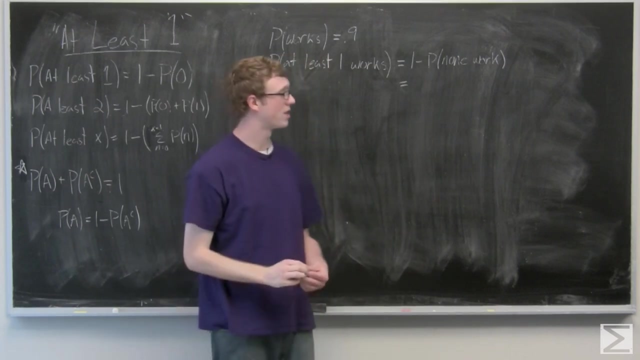 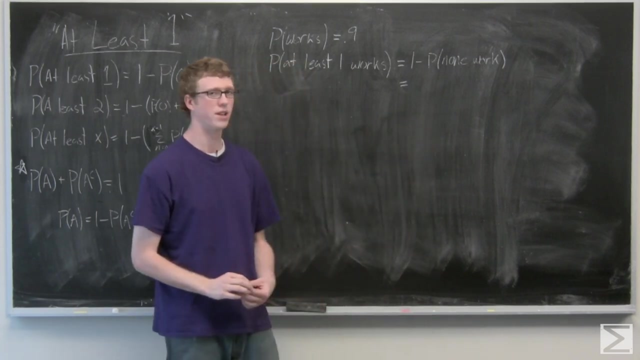 So that's going to be one minus the probability that none of them work. So that's the probability that none of them work, And the problem gave us that the reactors were independent of one another. so the probability that none of them work is The probability that a and B and C don't work, which is 0.1 for each. 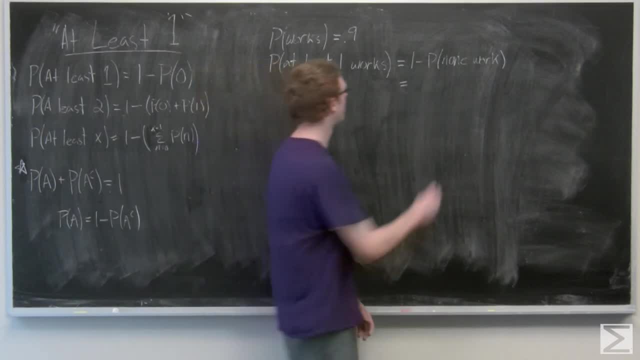 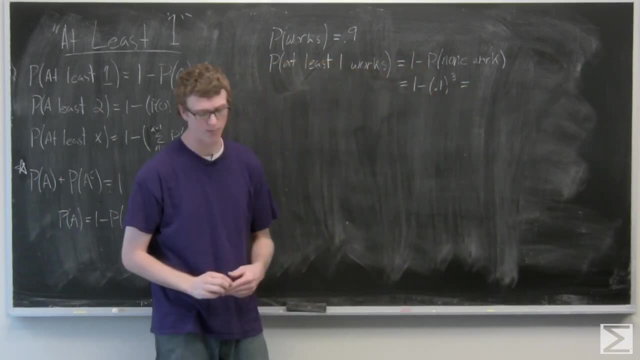 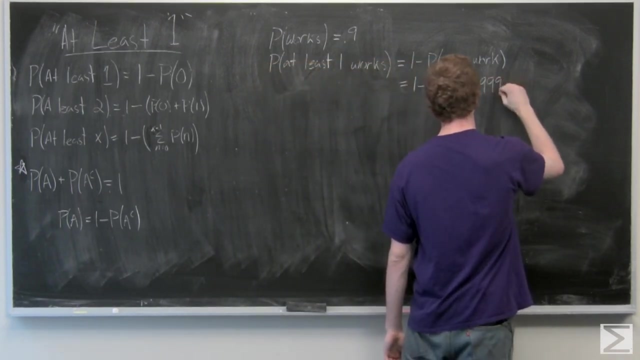 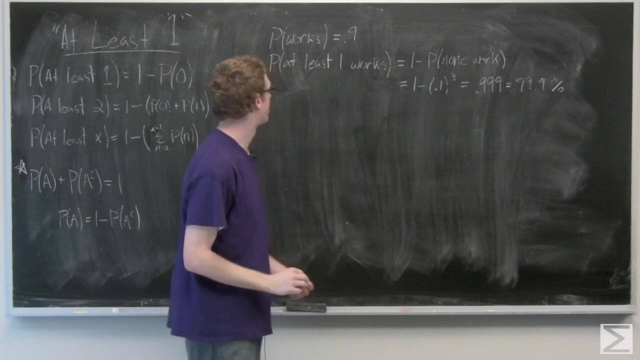 So we just have that probability is 0.1 cubed. Go ahead and plug this into your calculator calculator and you're gonna get 0.999, which Is a ninety nine point nine percent chance that at least one reactor works. so The scientists conclude that they have a pretty good chance of their chemical reactor working. 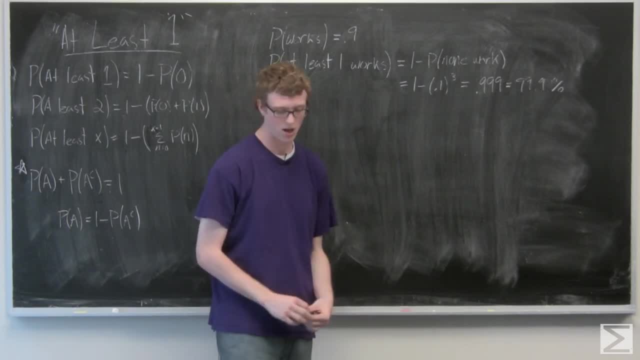 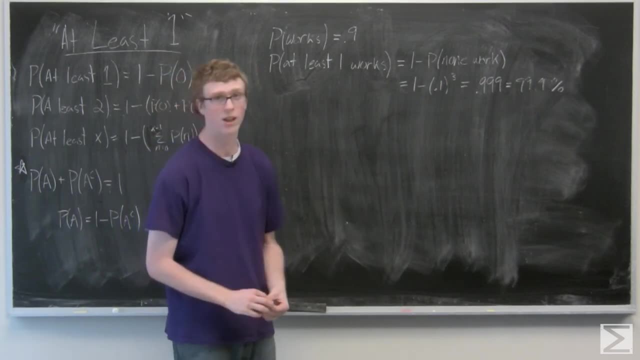 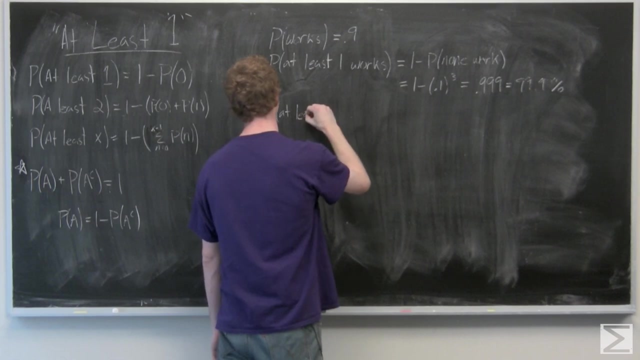 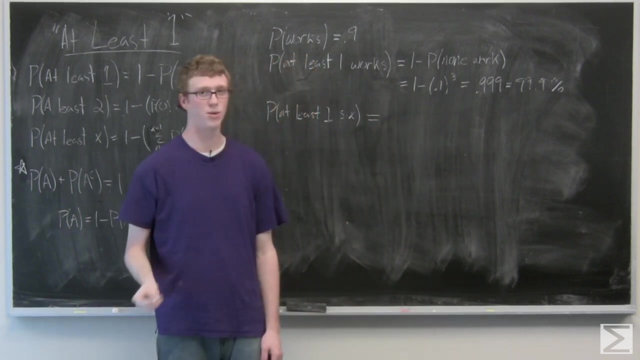 So now we're going to take a look again at some dice rolls. We're going to take a look at five dice rolls and the question asks: in five dice rolls, What is the probability that we get at least one cell Of six? Well, that's going to be one minus the probability that we don't get a six. 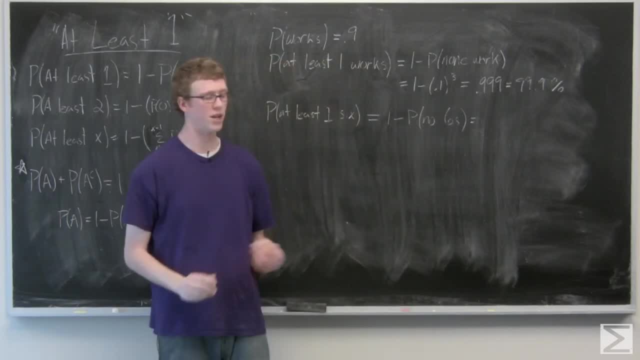 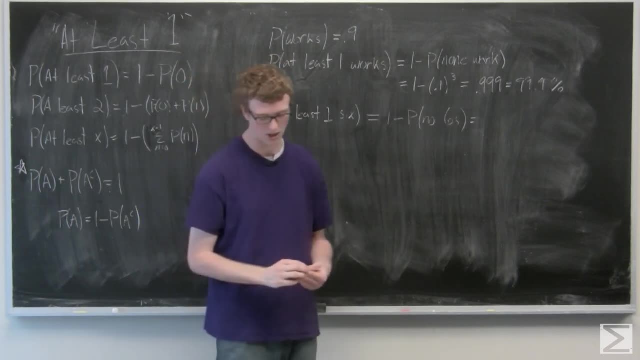 And Again, we're not told right away, But we know that the dice rolls are all independent because on each dice roll you can get one through six and the outcome of one doesn't affect outcome of the next roll. so we just have one minus and there's a five, six chance that you don't get a. 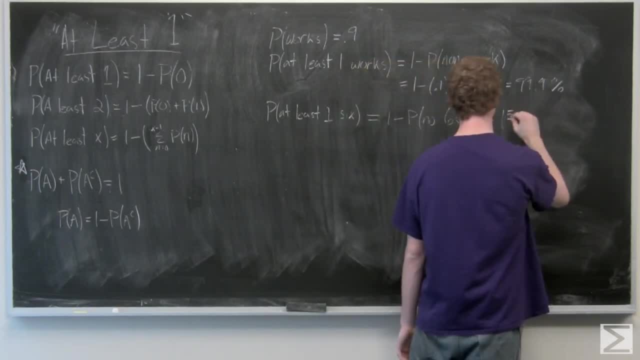 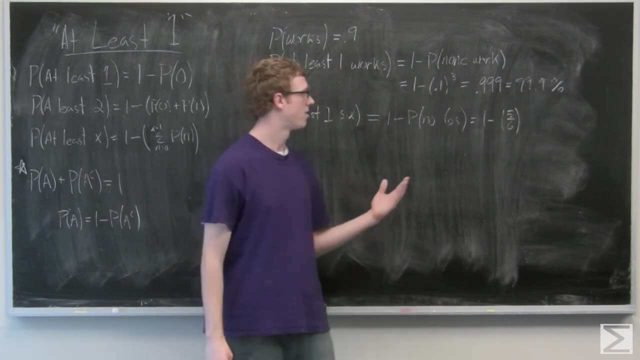 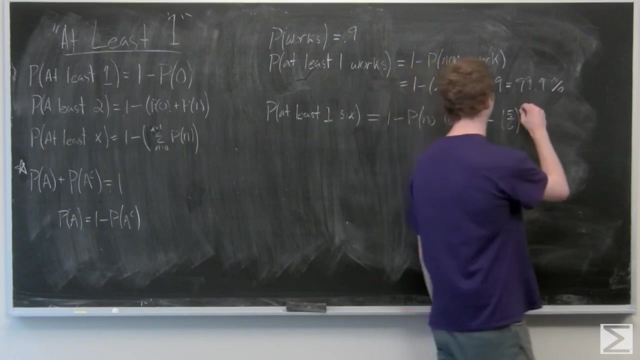 six and we said that there's five dice rolls. so, uh, probability that dice roll one and two and three and four. uh, don't get a six, is just gonna be five. six to the fifth: uh, go ahead and plug that into your calculator and you're going to get 0.598, 0.598. you can leave your probability as that, or 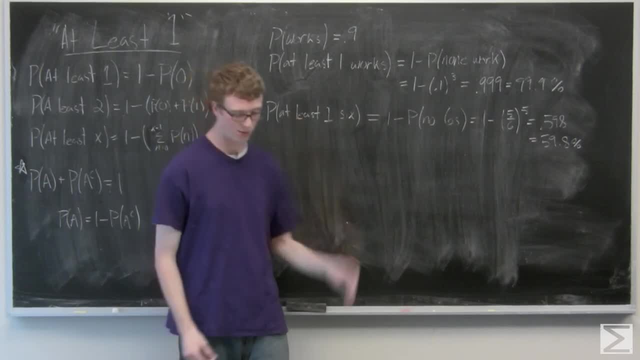 you can say that it's a 59.8 chance that we're going to get at least one six um the next one we have at a mathlete meeting. five men and three females attend and three are selected to compete in the next math competition. what is the probability that there's at least one female in the selection group? 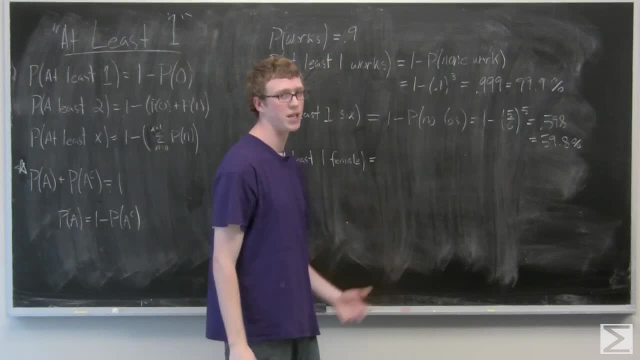 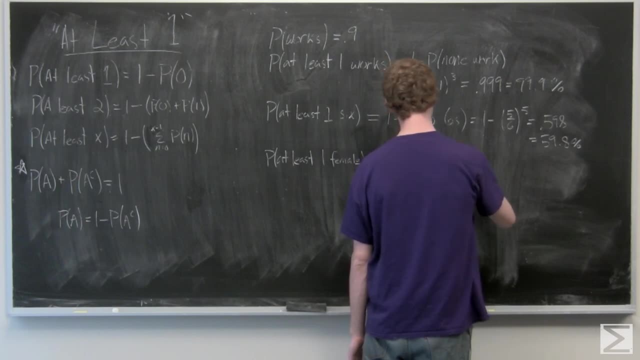 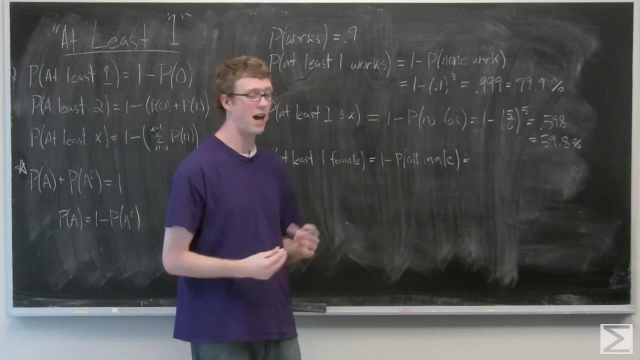 that's just one minus probability that there are no females, which is one minus probability that it's all males. and we have that. the probability of the first male is five out of eight. the probability of the second male, well we're. these are not independent trials, because if you take one man, then you have seven people left and 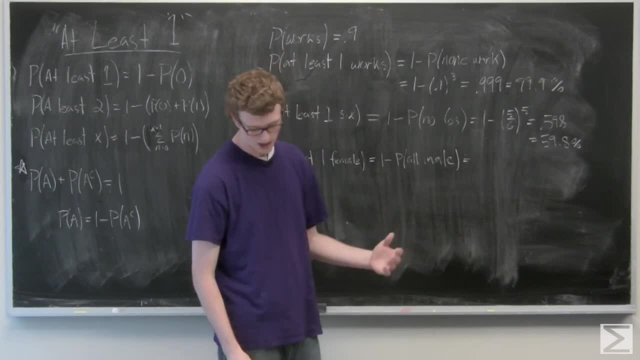 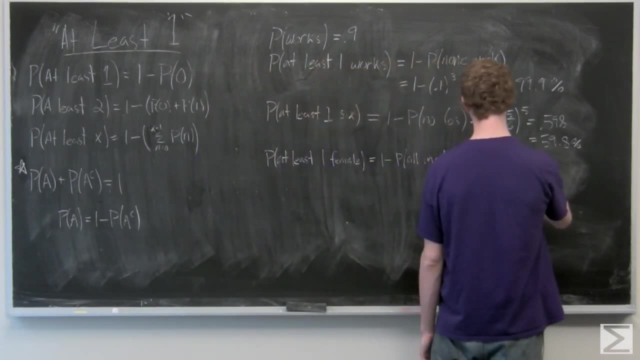 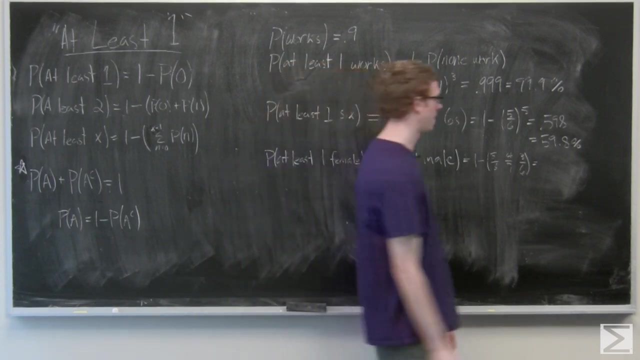 only four men, so it's one minus, uh, five out of eight times four out of seven times three out of six, and on the next round you're going to have um, And that probability is going to be 1 minus 5 out of 28,, or 23 out of 28.. 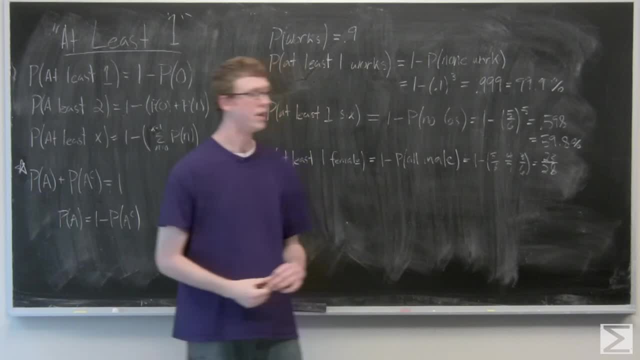 So that's the probability that at least one is going to be female, And the last one we're going to look at. a teacher gives a pop quiz with four questions that are true or false, And we have a student who has no idea what they're doing, so they guess at each. 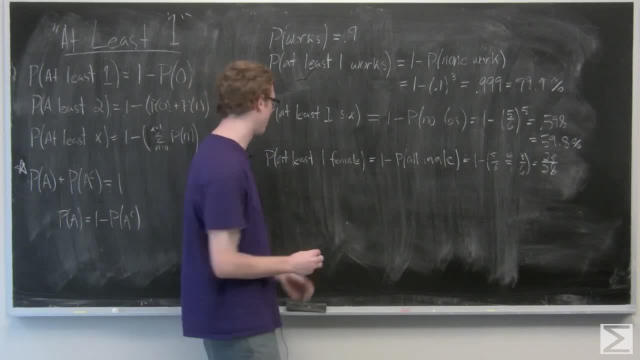 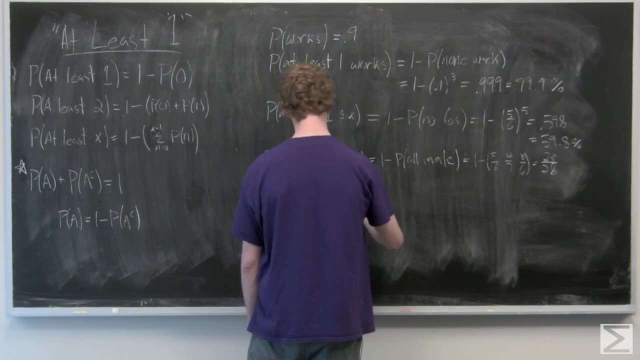 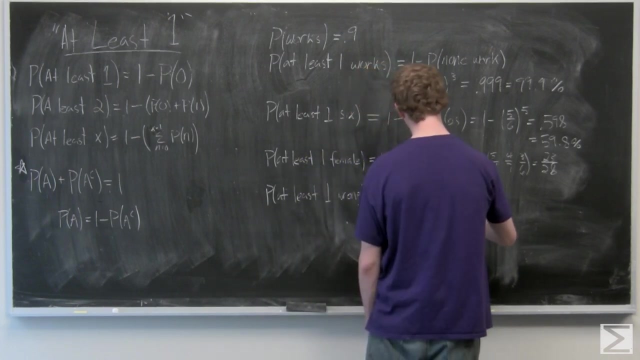 And we're going to find the probability that they get at least one wrong. Well, that's one minus the probability that they get them all correct, which probably isn't going to happen. The student has a one-half chance on each question. 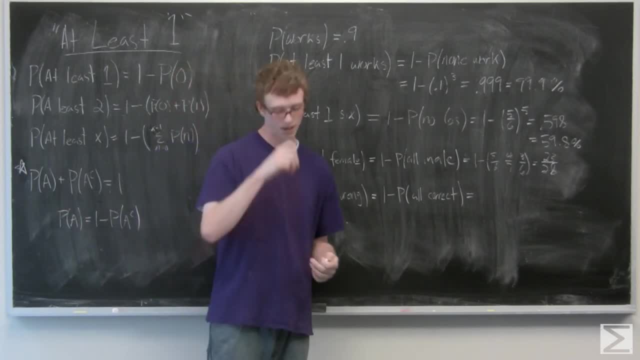 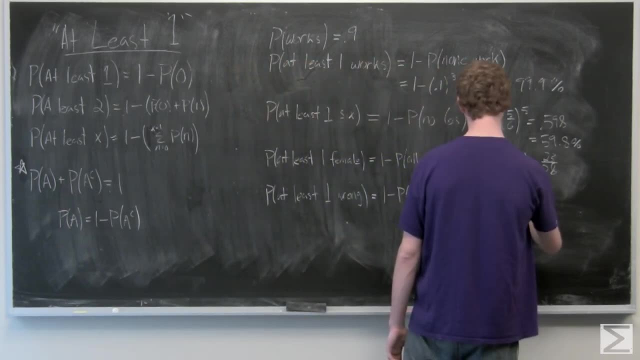 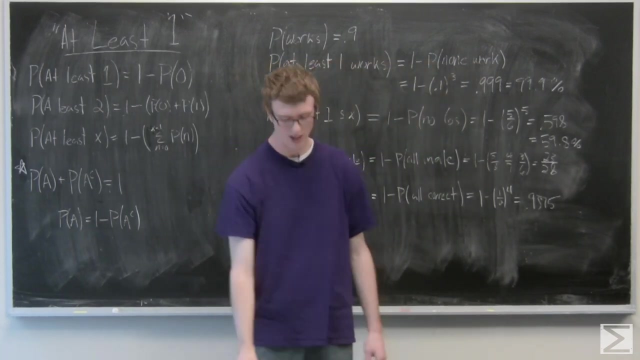 And each question is independent because they just guess on every question. So it's one minus one-half to the fourth And that's going to equal 0.9375.. So the student has a 0.9375 or 93.75% chance at getting at least one problem wrong.